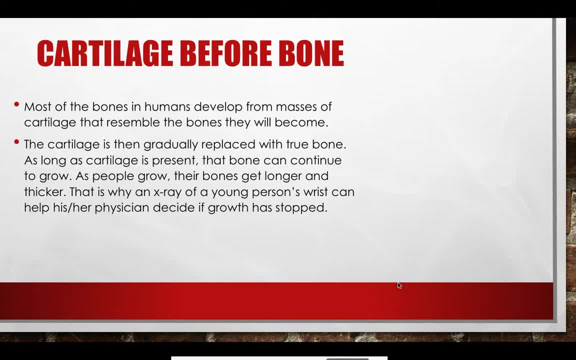 new bone. When we introducemes to bone compelx, inimal bones, we assume that these will freely develop and, as a result, their bones will resemble the bones they will become. Think of it almost like a blueprint that then the calcium deposits and true bone are grown onto. Now Our 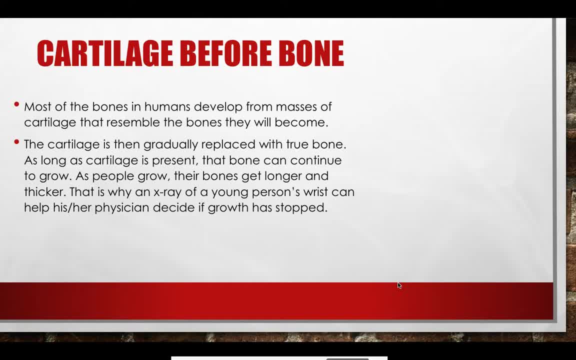 human adult skeletons still contain cartilage, such as between our major joints or in our nos or Our slavers. computers, But not Maple, would do such a thing. would we just become the prefrontal bone? nae, Yes, we could. The best I've ever done, cutting bones out where the cartilage goes, isأن a. 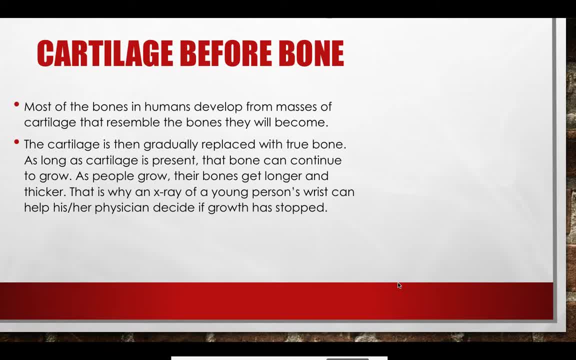 dessert. eventually we have the Deposan contact Now- in fact before that we would call thisмотрите, the brainic conversations. For with true bone, As long as cartilage is present, that bone can continue to grow. So as people grow, their bones get longer and thicker, and this is why x-rays can. 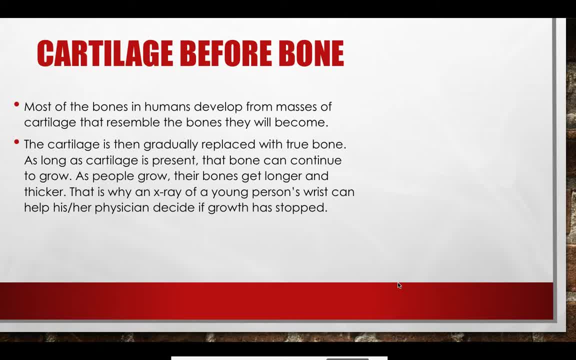 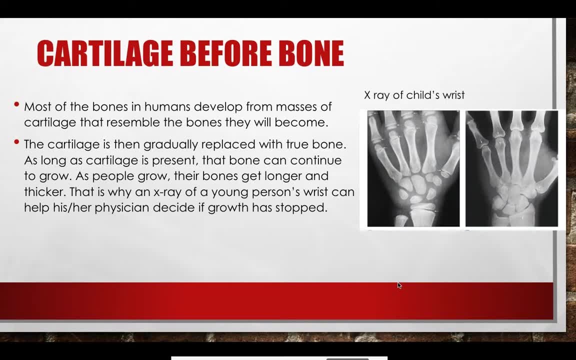 be used of young people's wrists to help tell a doctor whether growth is still happening or not. So take these x-rays on the side as an example. On the left hand side we have a child's wrist, and on the right hand side we have an adult's wrist. 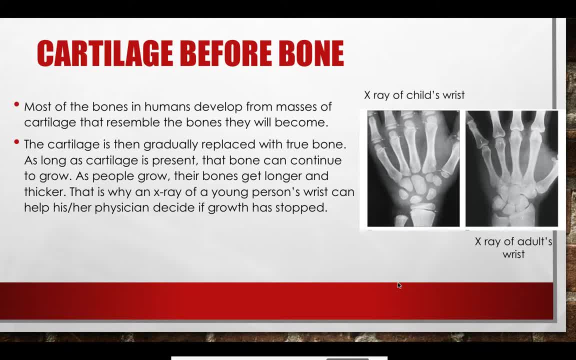 Now if you look at those carpal bones in the middle, you can see that there is a very big difference between the child and the adult. Child has a lot more space between those bones and the adults have very little space and are pretty much grown very close together. Now this shows that the child still has cartilage. 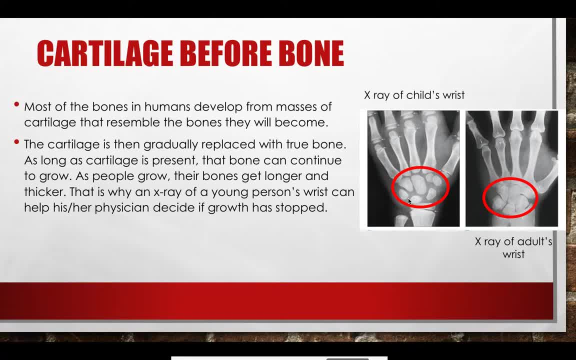 around those bones and room for growth right That cartilage will eventually turn to true bone, meaning that the child has more free space to feel and at least grow and develop move. So for the example of this, our� we have another big bone here Going down the right-hand side. here we have a. 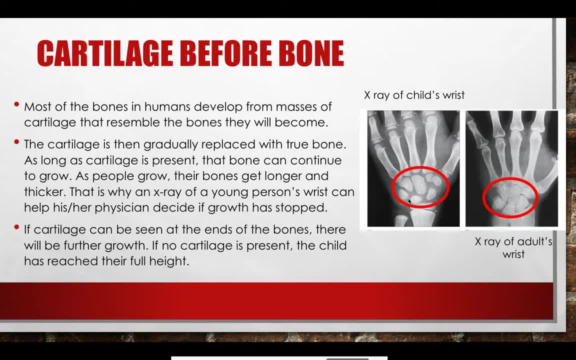 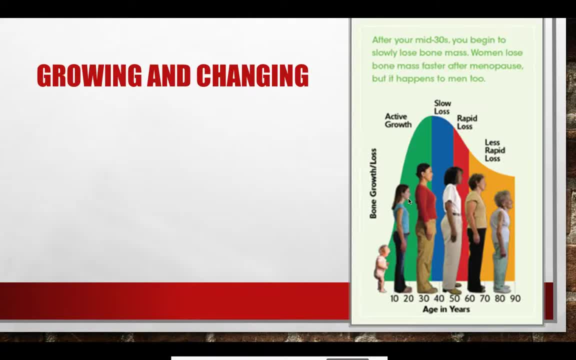 tiny bone knew skull and Alabama meat that are now going to have lower being and has not finished growing yet. However, if there is no cartilage present, that means that the child has reached their full growth Now in order for bones to grow all during life. 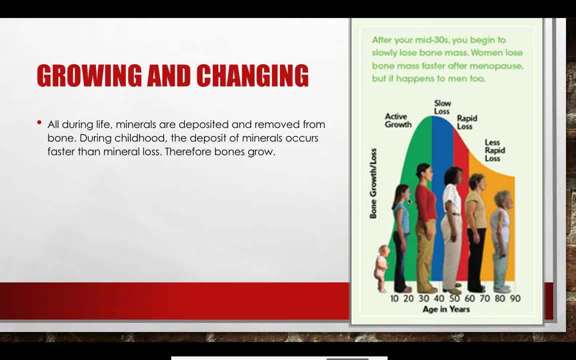 minerals are deposited onto that bone, They're also removed, interestingly enough. So during childhood, the deposit of minerals such as calcium occurs faster than mineral loss. Now this means that the bones are going to grow and get bigger, So this is why, as a child, you may have been told 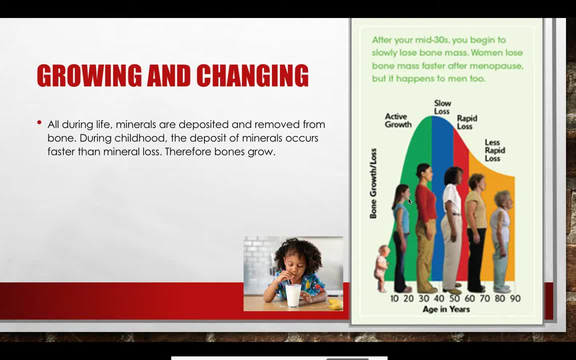 to drink your milk to make sure that you get that calcium and make some big, strong bones. Now this is actually really important because calcium is an important mineral that is stored in bones, so you wanted to make sure to have that in order to have adequate bone growth. 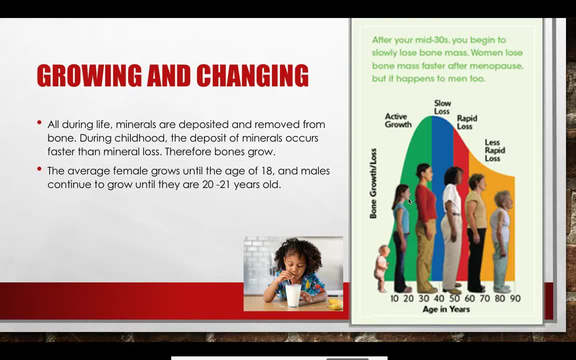 Now the average female grows until the age of 18, and males continue to grow until they're about 20 to 21.. After this stage the bones actually reach a kind of equilibrium From about the ages of 18 to 35, there is a balance. 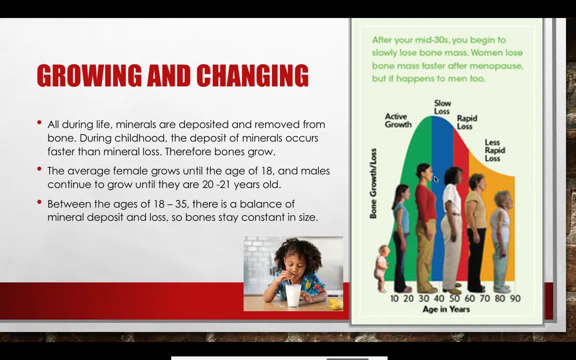 of mineral deposit and loss. So the bones stay the same size. However, if you look over in this graph here, you notice that suddenly there's a little bit of a difference. So suddenly after that age, that 35 mark. 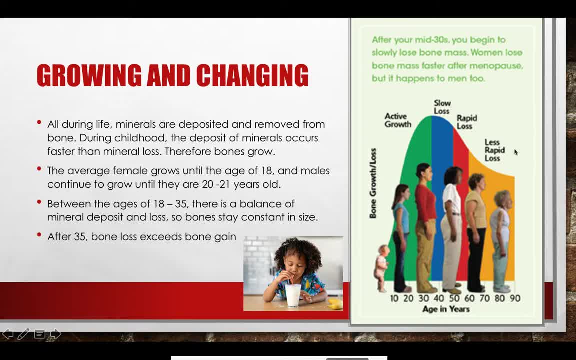 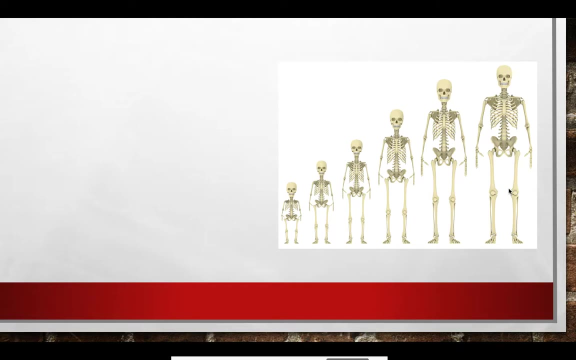 they start to decrease. So after 35, bone loss exceeds bone gain and this means that your bones may become weaker, it might be easier to break a bone or that you may see an actual decrease in the person's height. Now, one thing I usually ask my class to see is 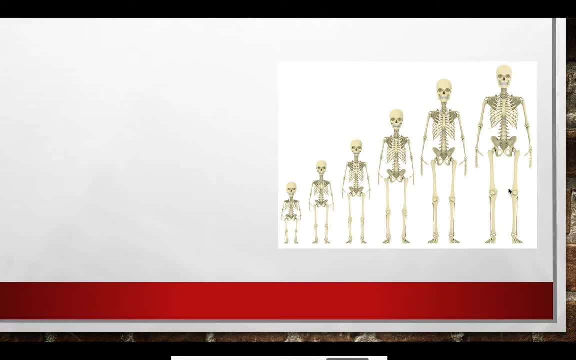 I get you guys to guess how many bones there are in a human body. So go ahead and take a random guess Or, if you're really quick, maybe try and count all the bones in this skeleton over here on the right-hand corner. Now, if you guessed 206, you're right on. 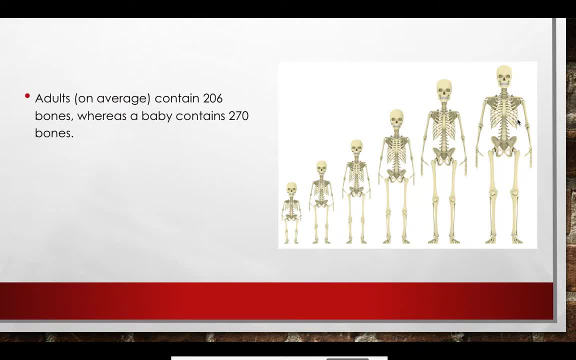 That is what the average adult skeleton has. Now you might be interested to find out that a baby actually contains 270 bones, and you might be thinking that's crazy. How can a tiny baby have more bones than a grown adult? Let me explain this. 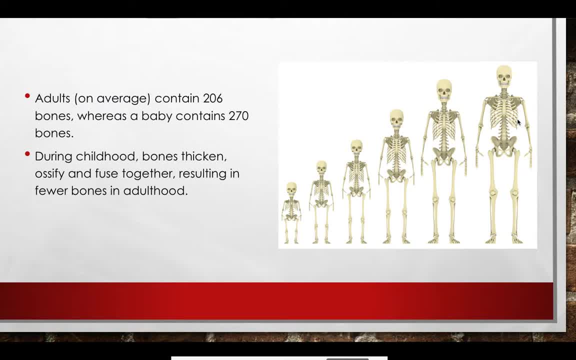 So during childhood, bones thicken and ossify and, most importantly, they fuse together. So this means that you have more bones as a baby, but as they fuse together and make one big bone, you actually have fewer bones as an adult. 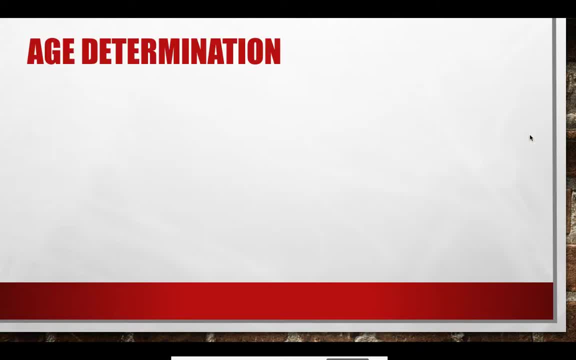 They're just larger, All right. so now that we know a little bit about bone growth, we can now use our knowledge to help and determine the ages of skeletons. Now, there's three major ways that we can do this. The most accurate estimations come from cranial sutures. 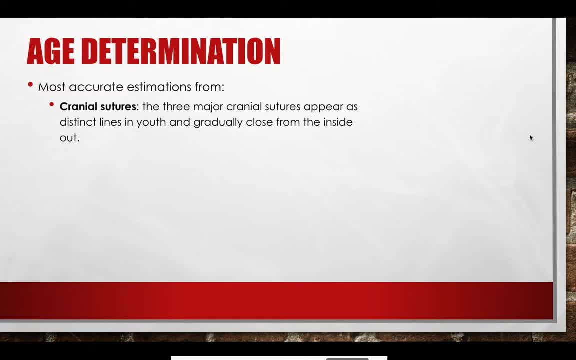 Remember, cranial meaning brain, so this is something to do with the skull. Now, these are three major cranial sutures that appear on on the human skull and they gradually close off from the inside out. We can use these to help determine age. 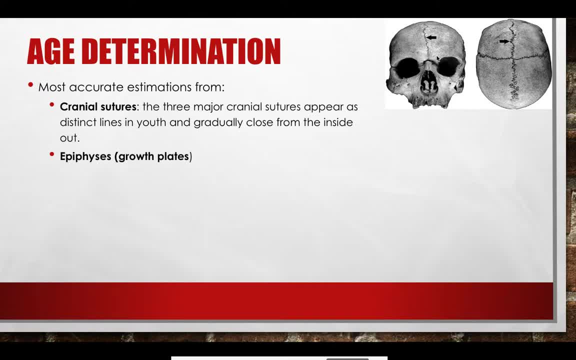 and we'll talk about it in a little bit. You can also use the epiphyses or the growth plates in a human bone, specifically your long bones. So right here is likely a femur right, And this is showing you the epiphysis, the end of that bone. 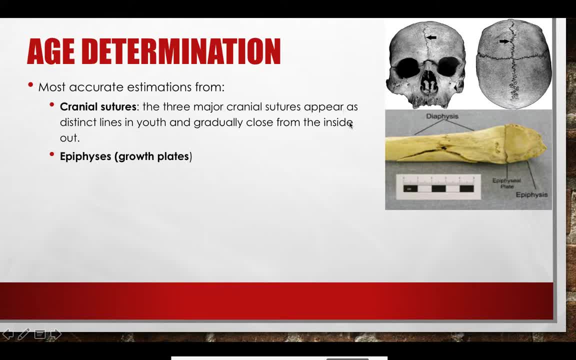 There's another one over here where the image is cut off. The epiphysis has a little section in it called the epiphyseal plate, also known as your growth plate. Now, by looking at the state that that growth plate is in, 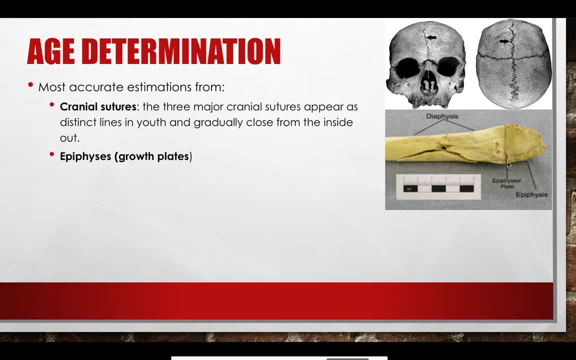 we can actually use that to determine the approximate age of the bone. The last option that we have is to use the teeth. Now, this is an image showing what a child's skull would look like with the bone, And this is a picture of a child's skull. 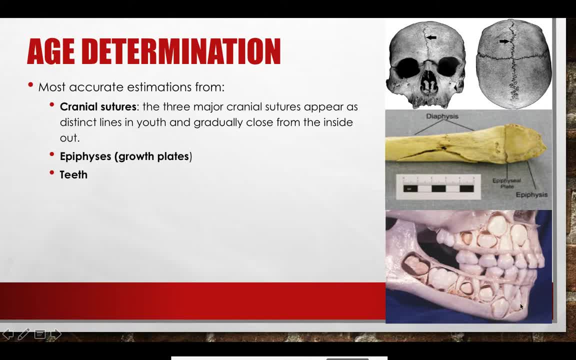 with those adult teeth still in the jaw. So by determining which teeth have emerged and which ones have not yet, we can get an approximate idea of how old that skull is or was when the person passed off. Now it's important to note that investigators 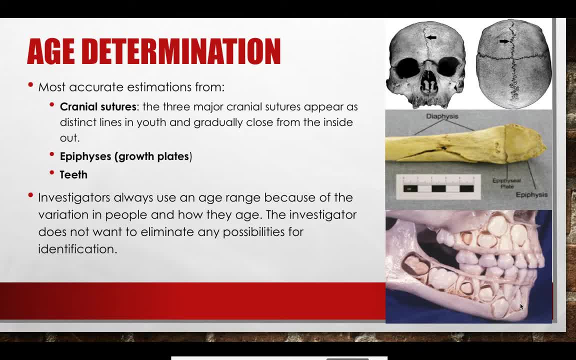 always use an age range when trying to determine a skeleton's age, And this is because of the variation in people, how they age. Everyone ages a little bit differently, So we don't want to give a definite answer of this skeleton was 16 years old. 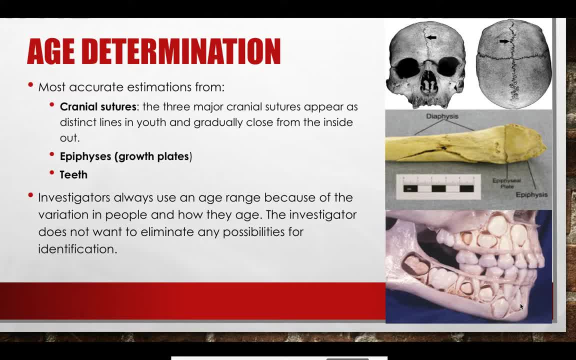 because maybe they were actually 20, but just had a slower growing process. So the investigator does not want to eliminate any possibilities of identifying a missing person. So they will always give an age range to try and make sure that they leave some possibilities open. 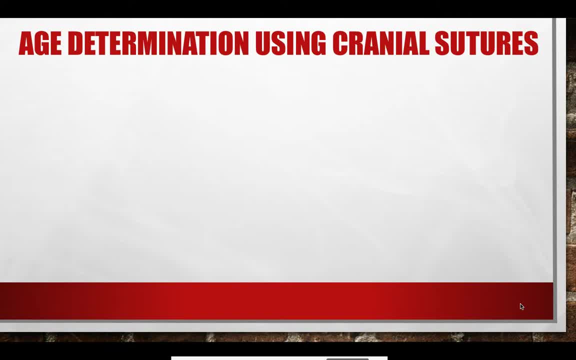 All right. so now let's talk about age determination when using cranial sutures, those lines on the skull. So think of sutures as immovable joints where bones are joined together And they're visible as seams on a surface. So think of, like the seam on your t-shirt right. 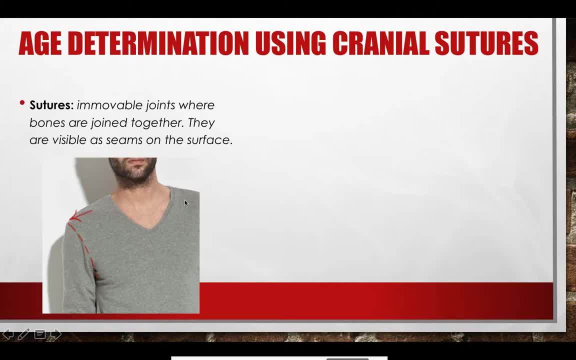 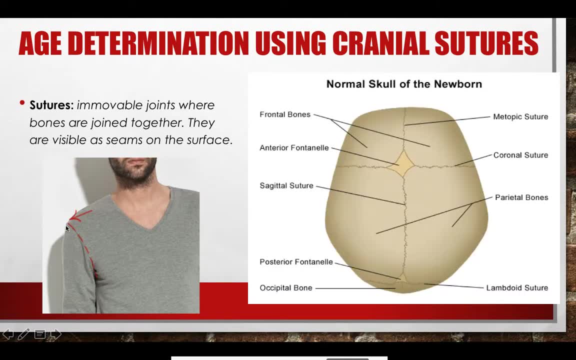 The one connecting that little arm hole to the body of your t-shirt. It's connecting those two sections and making it into one. That's exactly what the sutures are on your skull. They're connecting the many different plates or different bones of your skull. 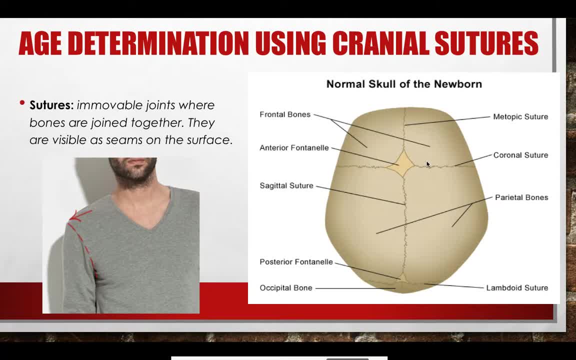 to make one smooth entire surface. Now, the three major sutures that we're going to be talking about is the coronal suture. Now, the coronal suture is located at the front of your head, horizontally, kind of like from ear to ear. 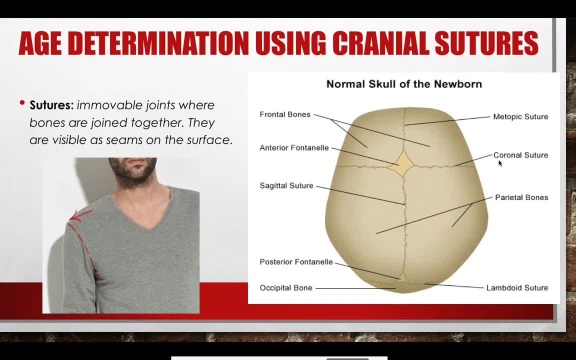 And the way I like to do it. I like to do it like this. I like to remember. this one is coronal, reminds me of crown, And if I was wearing a crown, I want it to be on the front, at the top of my head. 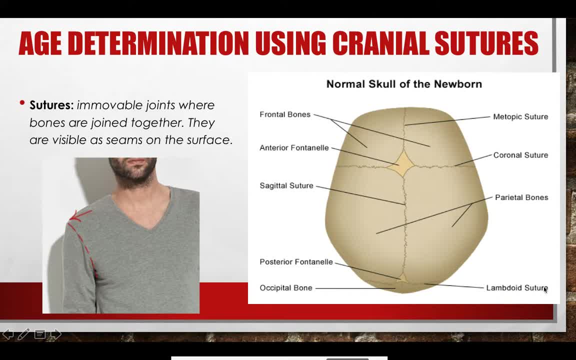 Another suture we'll be talking about is the lambdoid suture, And this is located at the very, very back of your skull horizontally. And the last one is your sagittal suture, which is running up and down across the top of your head. 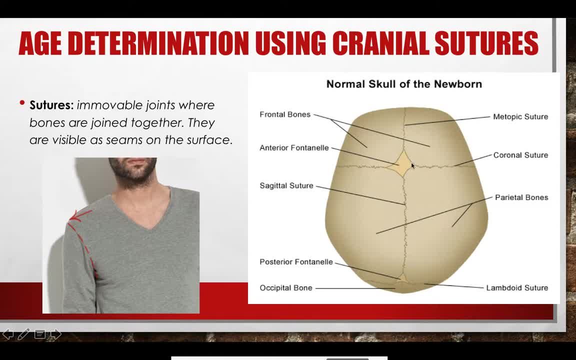 Now you may have also noticed in this image that there is a strange little hole in the middle of the skull, And if you feel your skull right now, the top right there, you notice that there isn't a hole anymore. That's because this image is showing the skull of a newborn. 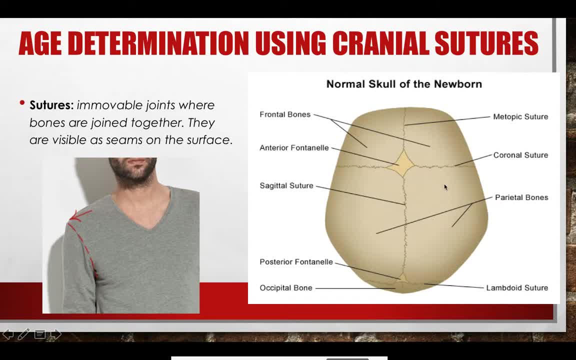 When a baby is born, those plates have not fully fused together yet, So there is actually what's called a soft spot on the baby's head for a little while, until those plates fully fuse together. Now this opening can be used to help estimate the age of a younger skeleton. 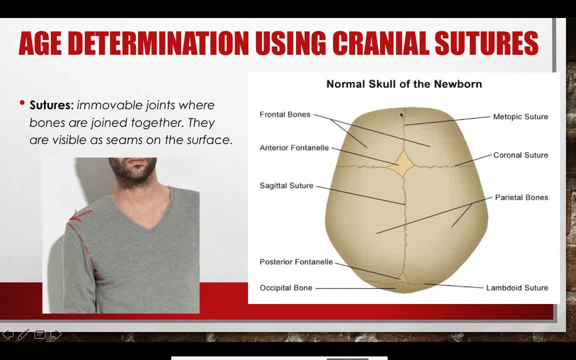 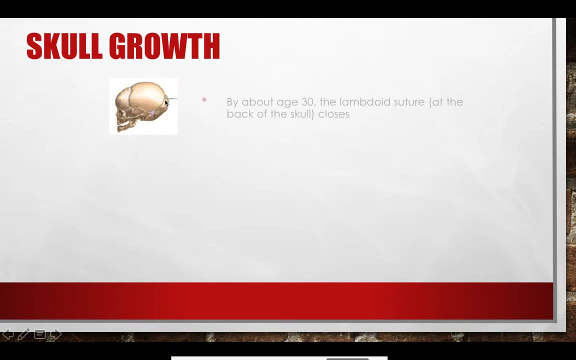 However, we can also use the stages of these suture lines and how far along they are in closing to help estimate age. Let me show you a little bit more Now that very back suture on the back of the skull here called the lambdoid suture. 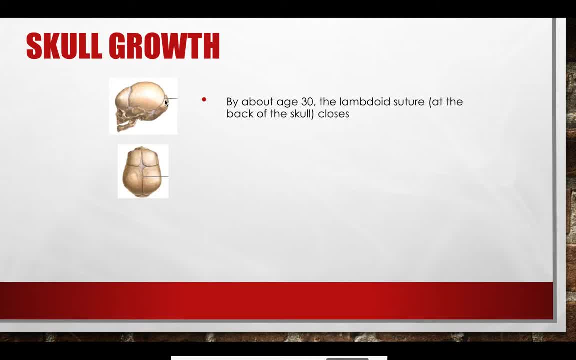 actually closes up around the age of 30.. The sagittal suture running from across the top of the skull, from back to front, closes by the age of about 32.. That front coronal suture we were talking about actually doesn't close until about the age of 50.. 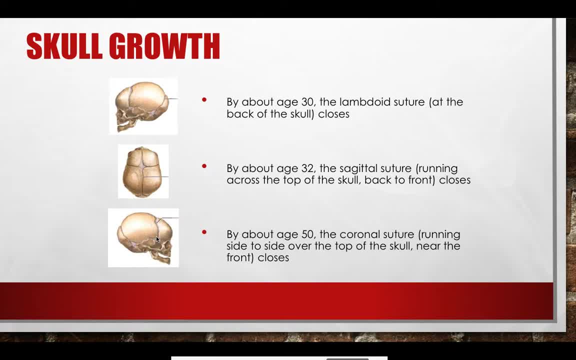 So by seeing the condition that these sutures are in on the skull, you can get a better idea of the age of the suture. So by seeing the condition that these sutures are in on the skull, you can get a better idea of the age of the suture. 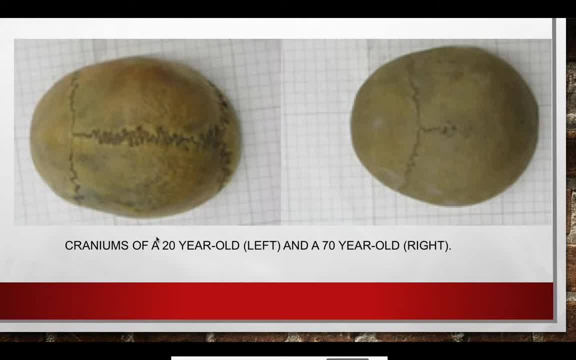 For example, here's two craniums. The one on the left is of about a 20-year-old, So you can see that those sutures are still very prominent, And on the right-hand side you have an 70 year-old individual. 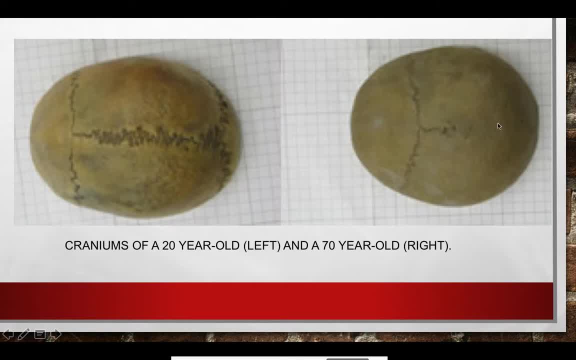 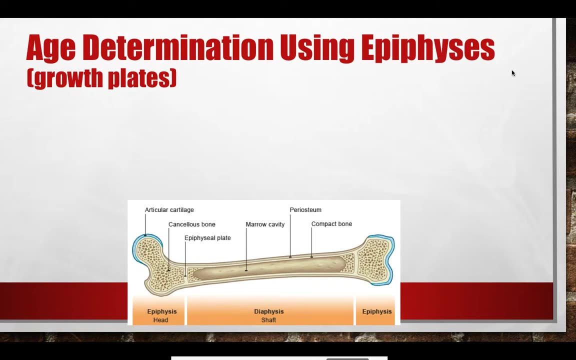 So you can see that those sutures are pretty much almost gone, especially for the lambdoid, one of the very back and completely closed up. Alright, so now that we have talked about cranial sutures, that is one way of estimating age. The other is by using those growth plates, So the long bones, 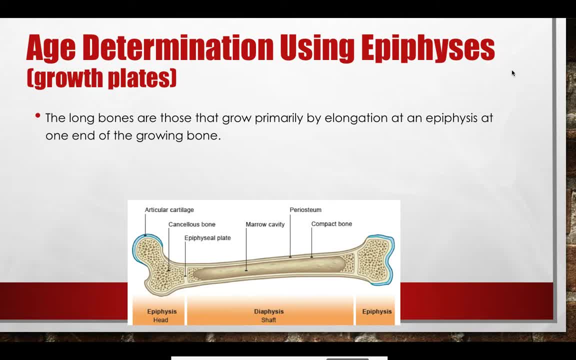 that are used Alright. so now that we've talked about how to use cranial sutures to estimate age, we're now going to talk about growth plates. The long bones are those that grow primarily by elongation at the epiphysis, at one end of the growing bone, So on either end of your bone. 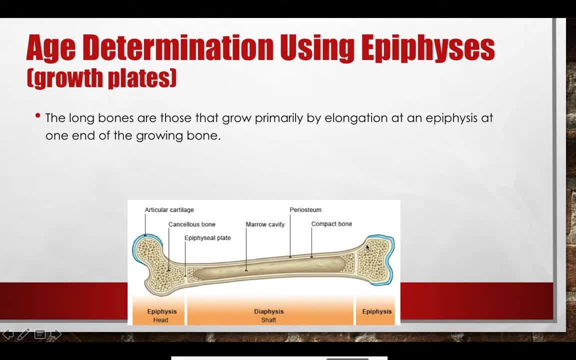 you have this kind of- you know- bumpy region and that is where your bones connect to other areas of your body. This is called the epiphysis, Now the region in the middle. the diaphysis is that central area where marrow is stored or where blood cells are created And in the ends, 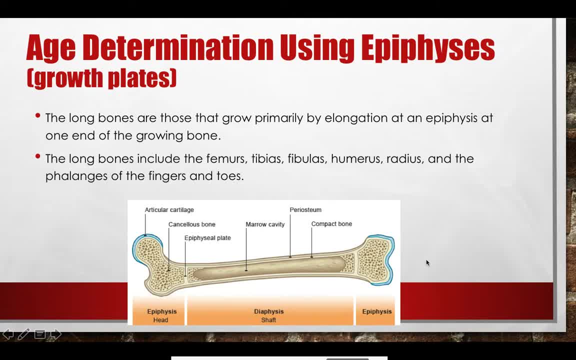 you also have bone growth happening, So the long bones typically include your femurs, tibias, vivias, humerus, radius, ulna and the phalanges in your fingers and toes. Now, if you're having trouble remembering where these bones are, I really suggest that you go back to Friday's video. 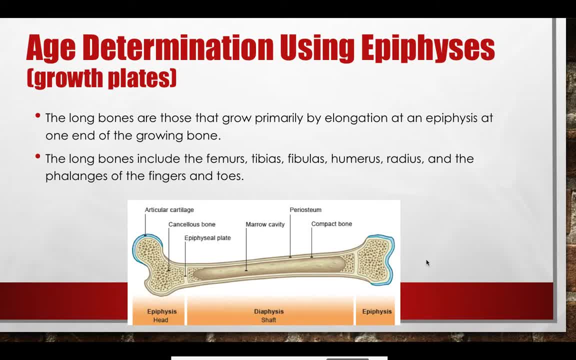 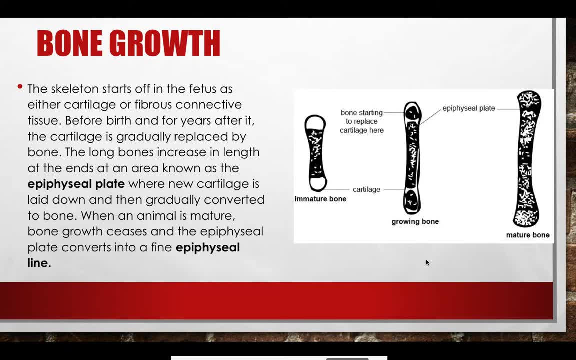 or try and re-label your skeleton diagram, Alright. so, as we've talked about, the skeleton starts off in the fetus as either cartilage or fibrous connective tissue. right, You have that cartilage outline of what our true bones are going to look like. So before birth and years afterwards. 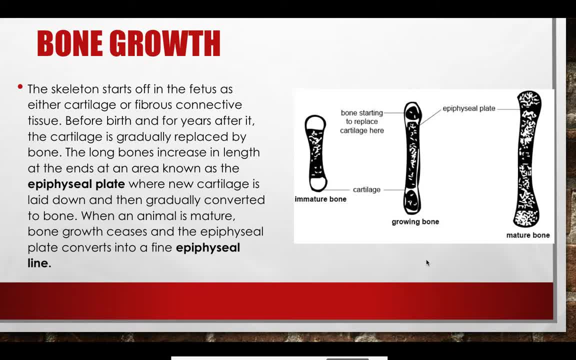 that cartilage is then gradually replaced with bone. So what happens is that the bones increase in length at the ends, at the area called the epiphyseal plate. So, for example, this is an immature bone that has cartilage on either end. Now, as it grows, 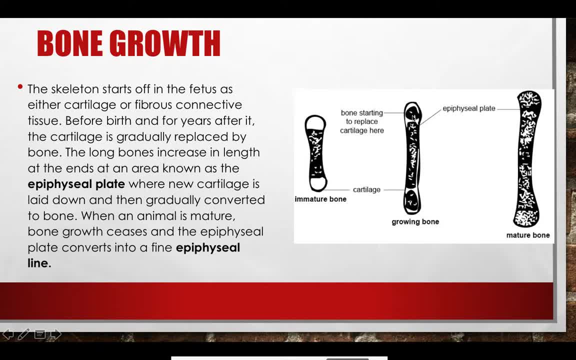 that growing bone actually starts to grow at either end, leaving us with this funny little plate of cartilage. So as long as there's that new cartilage being produced, that bone will continue to be converted from that cartilage and that bone will continue to grow Once an animal is mature. 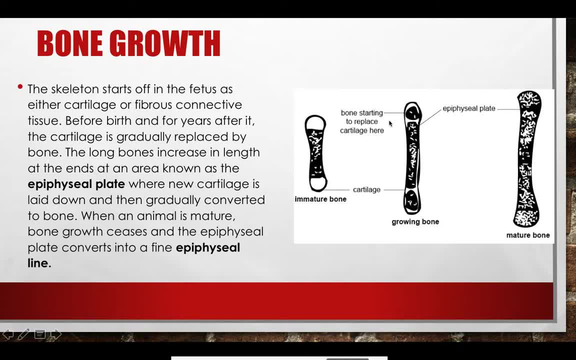 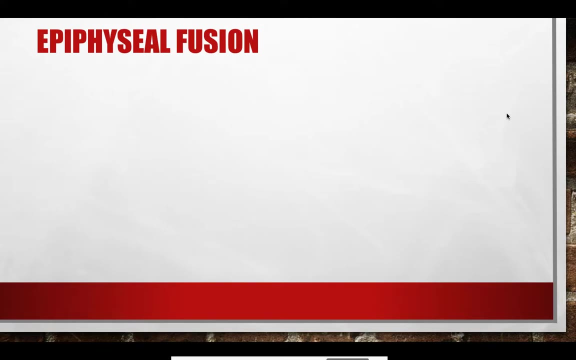 that bone growth stops and the epiphyseal plate converts into a fine epiphyseal line, which is very noticeable. Instead of being this large cartilaginous plate area, you now have a very fine bone line, So that can be helped to use during examination of a bone to see if that individual was still 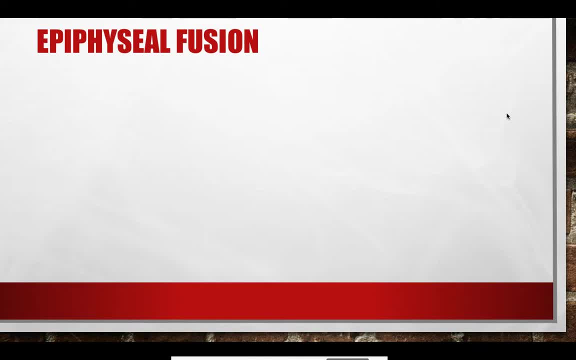 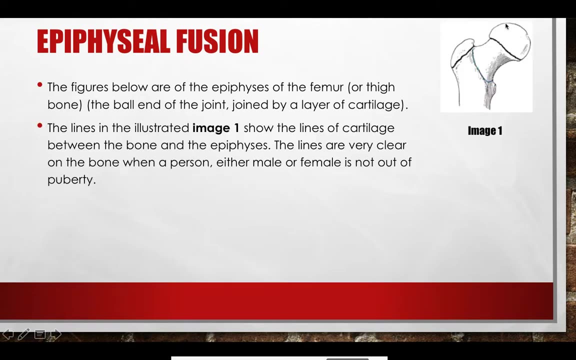 growing or not. We also can talk about epiphyseal fusion. So in the images I'm about to show, this is showing you the epiphyses of a femur or that thigh bone. So you can tell right here this is that joint ball and socket area that would be connecting into the hip. 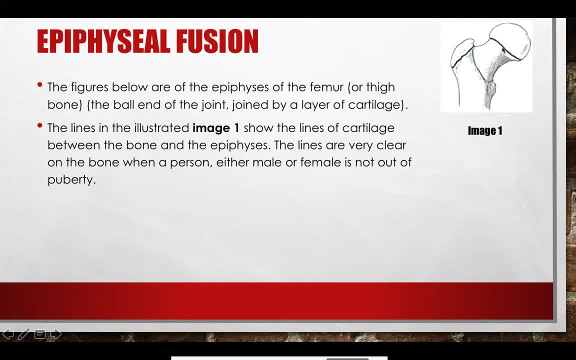 Now, if you see these very defined lines of cartilage between the bone and the epiphyses, that is showing that the bone is still growing. The person hasn't gotten out of puberty yet, and so their bones are still typically growing at that point. If you were to see a bone like this: 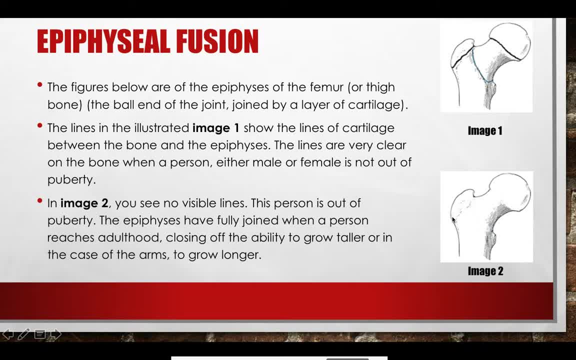 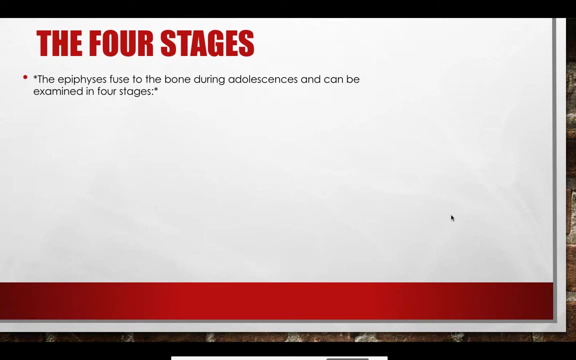 where those lines are not as defined and it's more just smooth bone, that is indicating that there is no more cartilage and that their ability to grow taller or longer arms is done. That person has stopped growing. Now we can also talk about the four stages of bone growth, and these really help in determining 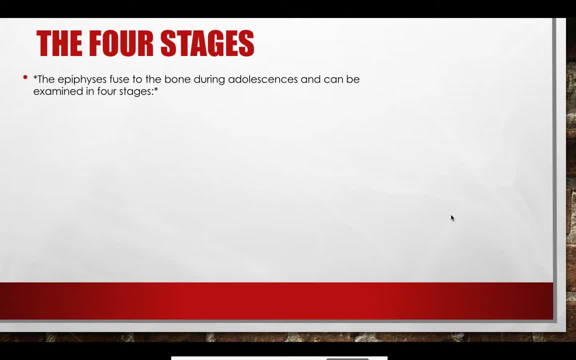 the age, especially of like adolescents, and determining whether their bones have finished growing or not. So our first stage is called Stage 1, and it says non-union with no epiphysis. So this means that the growth plate has not even started. 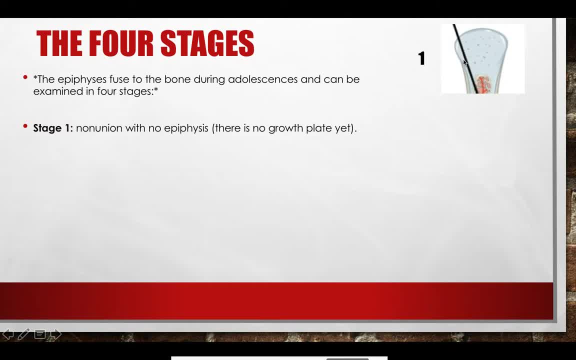 yet Typically looks like this: It's a lot of just cartilage at the end. so this would indicate a very young individual, especially if there's no growth plate yet. Stage 2, non-union, with separate epiphysis. So the growth plate has formed but it's not attached yet. 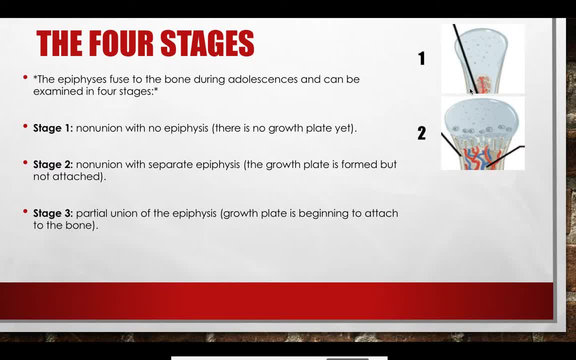 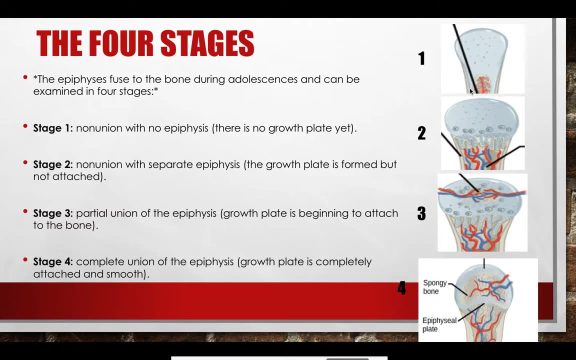 Stage three is partial union of the epiphysis, So the growth plate is now beginning to attach to the bone. And lastly is stage four. This is complete union of the epiphysis, meaning that the growth plate is completely attached and smooth. You can definitely tell here that that 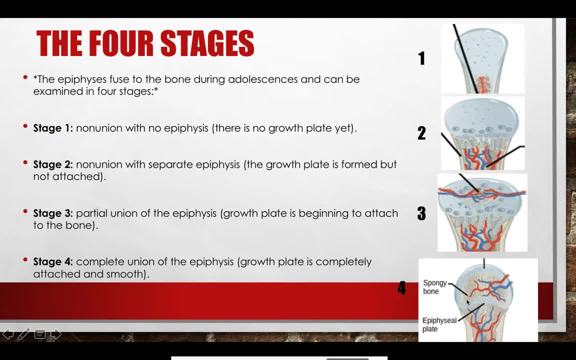 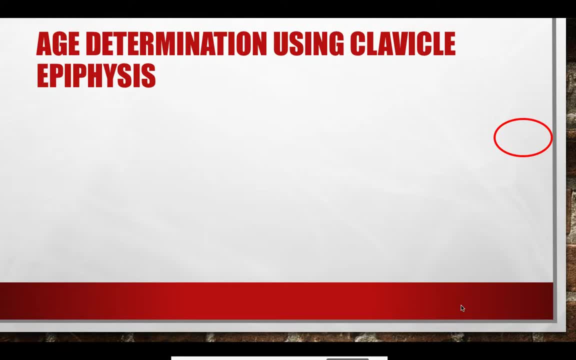 growth plate is very, very smooth indeed And that bone can continue to grow there All right now. the reason that I had to talk about those four stages is because we can use those four stages to estimate how old that child or individual was. Let's use the clavicle. 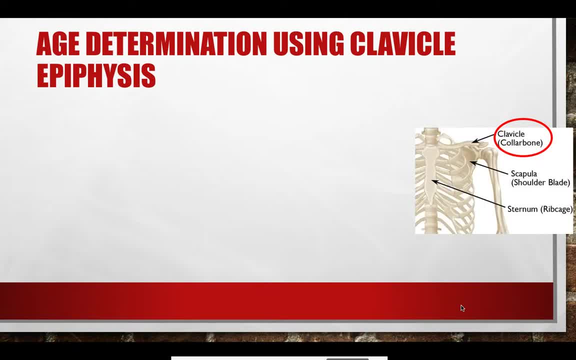 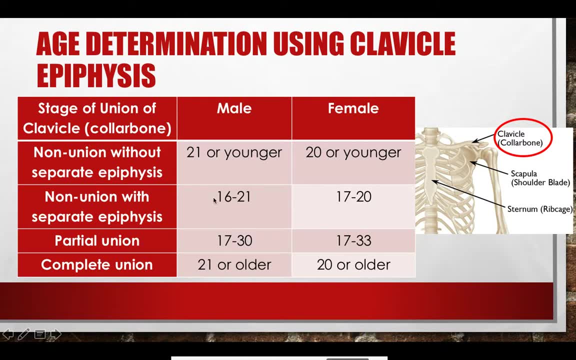 as an example, Clavicle is your collarbone. If I were to examine this in a skeleton, I can use those four stages to actually estimate how old the individual was. Now this differs between males and females. However, it does give us a decent idea. 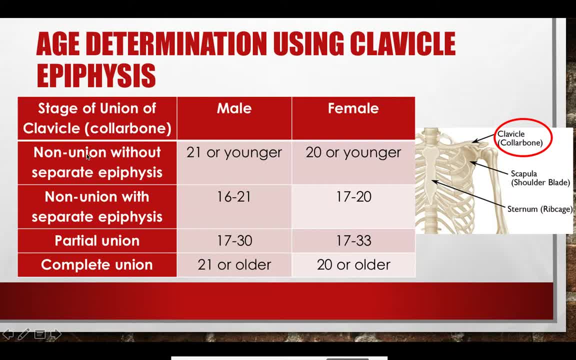 So by having nonunion without a separate epiphysis, we know that the individual was 21 or younger. If there was a separate epiphysis, the individual was probably a young adult to a teenager between 16 to 21. A partial union indicates that they're. 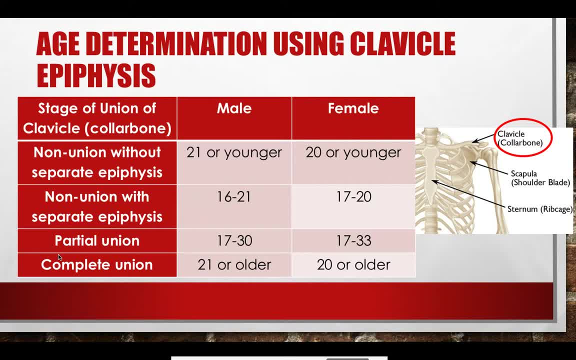 probably about 17 to 30. So they're possibly a little bit older now, And complete union means that they were 21 or older Now. I know that these age ranges are pretty large. However, by comparing the growth stages of multiple bones in a skeleton, you can see that the growth stages of the skeleton 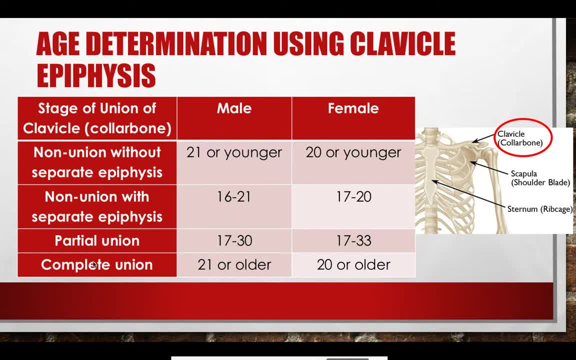 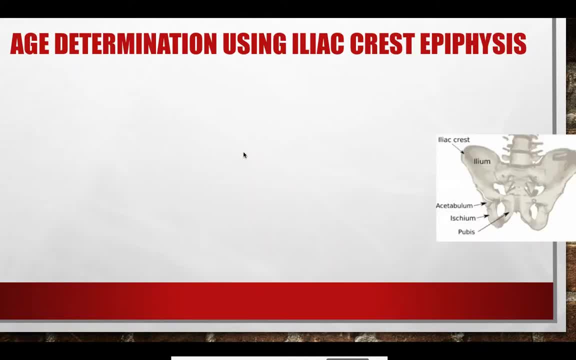 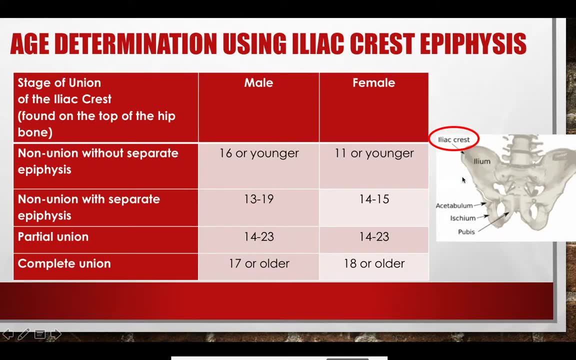 you can get a better idea. For example, these are the age ranges from just the clavicle. I could also have found maybe a hip bone at my crime scene, And by using my iliac crest to that edge of my hip bone I can figure out a variety of different things, especially. 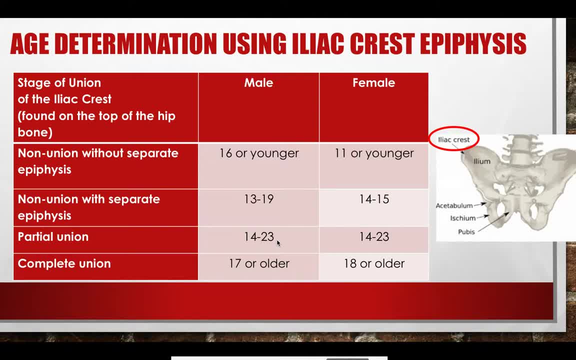 if that skeleton was younger. So in this case, if there's no union and no separate epiphysis, that means that the individual was 16 or younger for a male, or even 11 or younger for a female. Next stage for stage two. if I find that my iliac crest is at stage two, 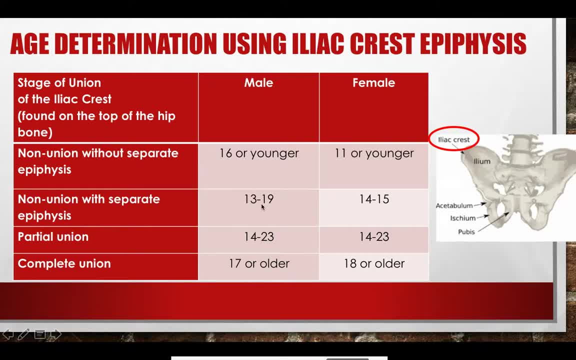 that means that now my male is somewhere between 13 to 19, or a very short range of 14 to 15. for females, Stage three would indicate anywhere from 14 to 23.. And a complete union is now definitely indicating an older individual somewhere between 18. 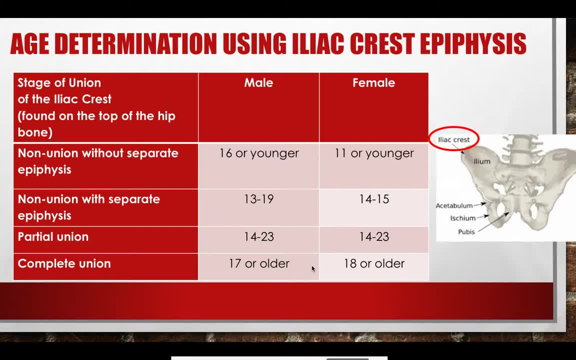 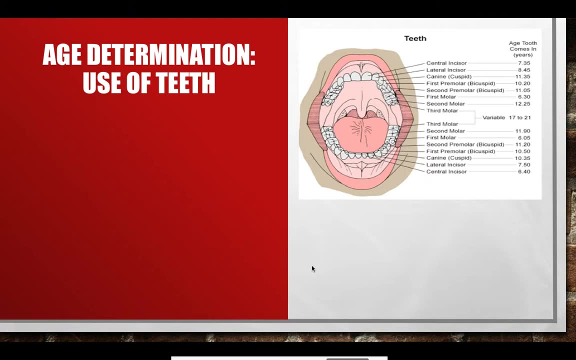 and above, So this can also give you a good age range for some younger individuals or skeletons that you may find, Hopefully, not All right. So now that we've talked about how the growth plates in bones can help indicate age, we're also going to talk about teeth. 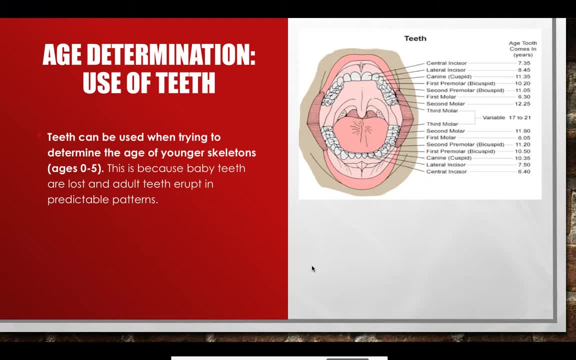 Now teeth can be used when trying to determine the age of younger skeletons, typically between the ages of zero to five, And this is because baby teeth are lost and adult teeth erupt at predictable patterns. If you think back to the first tooth you lost, it was probably your central incisor. 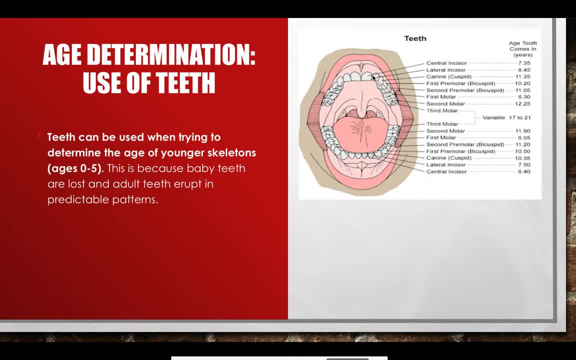 also known as your front tooth, And you were probably between the ages of six and seven. Speaker 2: You probably looked a little bit like this, either going into kindergarten or grade one. So by knowing the predictable pattern we can actually determine the approximate age of an. 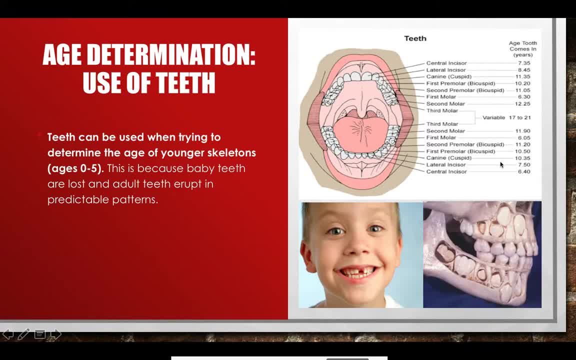 individual based on which teeth are remaining in their jaw and which ones have erupted and are now in the mouth of that skeleton. Now it is much more difficult to determine age of older skeletons by using teeth, because they don't have baby teeth anymore typically and all of their 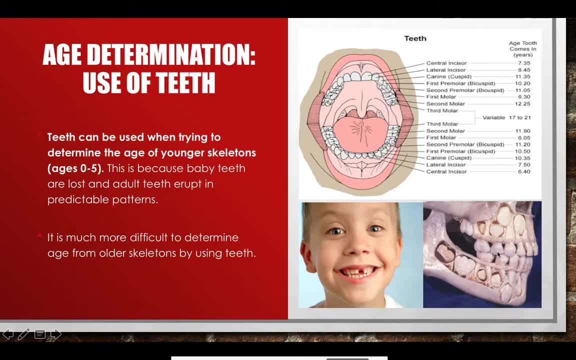 teeth have erupted out So you could use regular wear and tear. however, this isn't going to give you a reliable response. Usually, with older skeletons of adult ages, you're going to have to use other bones as well to help confirm age. You can't just rely on teeth. All right. 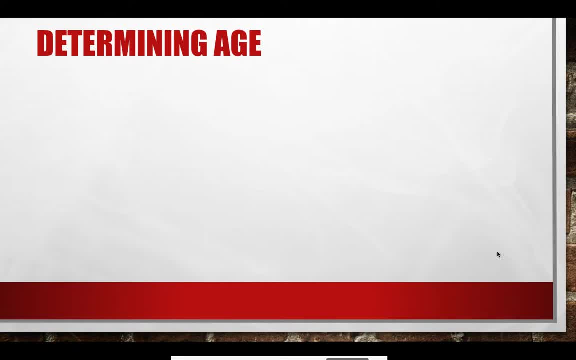 so when determining age, we have a few different options and, based on the age of the skeleton, certain options are going to be better than others. So for skeletons that are ages 0 to 5, teeth are the best indicator of age, and this is because baby teeth are lost and adult teeth erupt. 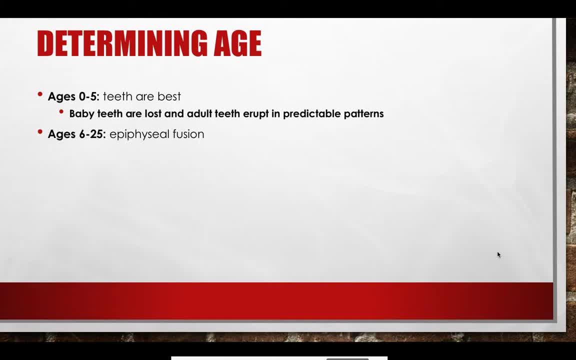 at predictable patterns Between the ages of 6 and 25, the age of the skeleton is going to be the most likely indicator of age. So, for example, if you have an epiphyseal fusion, that growth plate in your bones is one of the more likely indicators of age. Now it's also 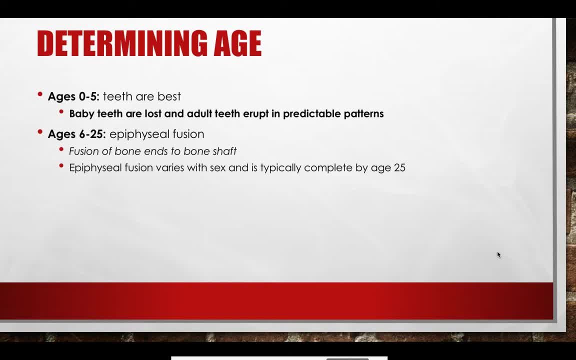 important to remember that this does vary depending on your gender, but is typically complete by the age of 25.. So this means that the ages between 25 and 40 are quite difficult to determine because there's no specific indicator to help tell age, just by visibly looking at them anyways. 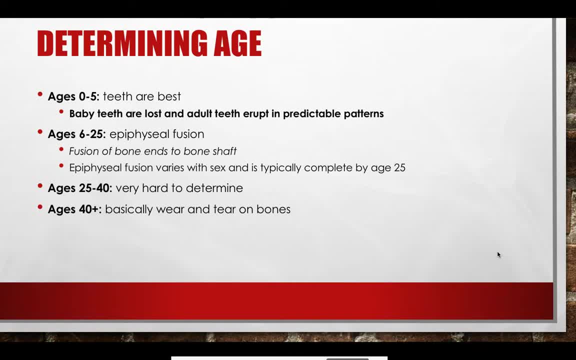 Now above the ages of 40, it can also be quite difficult. However, there may be some regular wear and tear on those bones or they may have also started to reduce in size, So you can use that as well as arthritis, breakdown of pelvis, things like that. 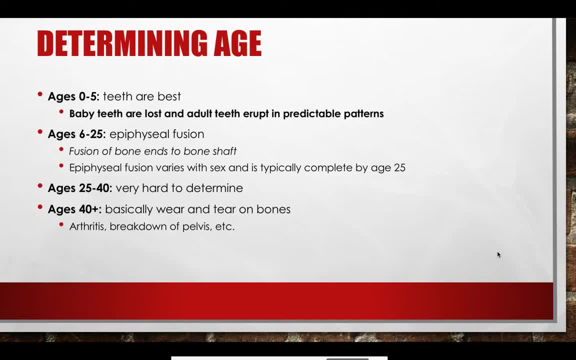 All right, everybody. I hope that you enjoyed this video And if you have any questions, please email me. I am going to be attaching a short little question sheet to this video And that is to be assigned for tomorrow's work. However, if you're feeling like doing it today, 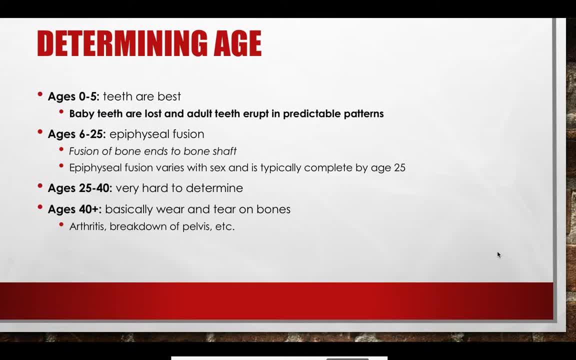 because you just watched the video. I'm totally fine with that, and go ahead and get Friday's work done a little early. Have a great day, everybody. Bye-bye.